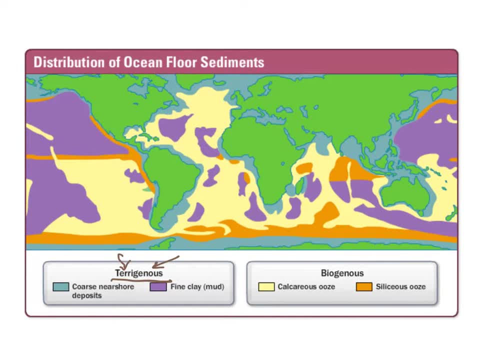 So these are going to be the ones that are made up of rock, basically, And what we have is two different kinds and it's based primarily on the texture or the size of the grain that makes it up. We're going to have these coarse near shore deposits, and that's going to be things. 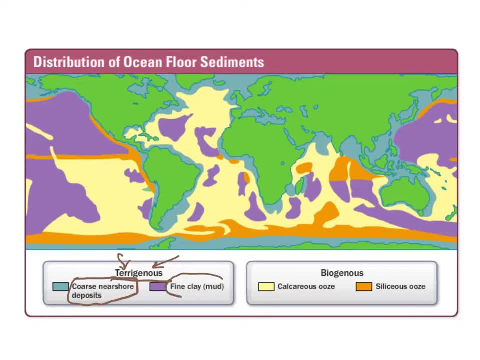 like sand and gravel, And then further out we'll have this fine clay and mud type of sediments as well, But these are teragenous in nature, so they come from rocks. It's the base up, ground up, minerals and rocks and things of that nature, and that's what makes this sediment. 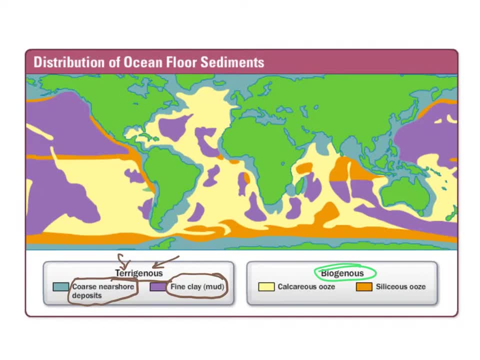 Now the next type of sediment is what we call biogenous. Biogenous means that it comes from life. So there's two primary types of biogenous sediments, and it's going to be based on the material of them. We have silicaceous ooze and then we have this calcareous ooze. The calcareous ones are going to 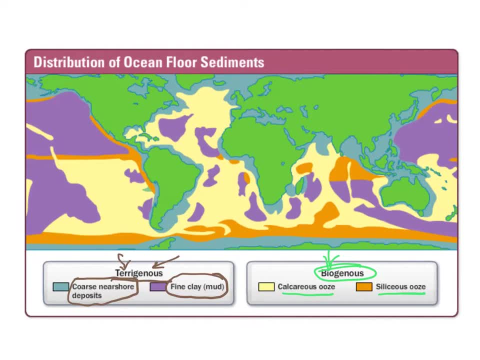 come from shells, So it's calcium carbonate like you'd see in a seashell, and are in corals, And what you're going to see is this material is just kind of eroded away, weathered down, and it's made up of these materials. We can also have a silicaceous ooze which is going to come from the. 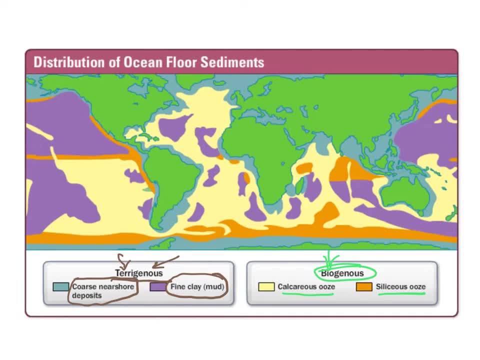 shells of diatoms, which are microscopic, little marine organisms as well, But instead of having a calcium carbonate shell, it's one that's primarily silicone. And then the third type of seafloor sediment is what we call hydrogenous, and that's going to come from the water, And this 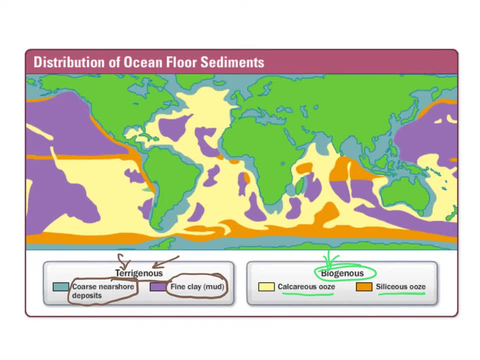 is where we're going to see things like our manganese nodules that are going to form- that you'll learn about a little bit in our lesson- And these are going to be these precipitates that come from the water, So we can have stuff that's trapped in the water and it'll precipitate. 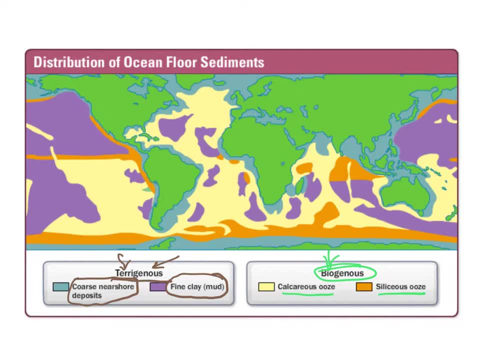 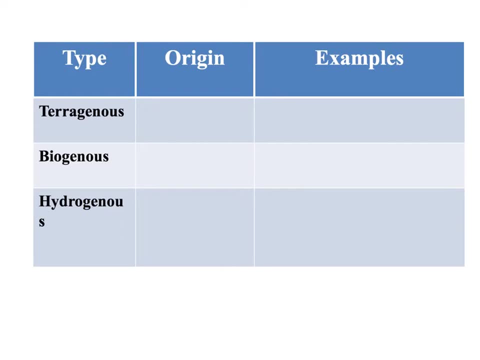 outwards, So it comes from the water, hence the term hydrogenous. Okay, so just to summarize these, let's take a look real quickly. We have our three different types. We have our terrigenous sediments. The origin of that is going to be land and those are going to be primarily from the rocks. 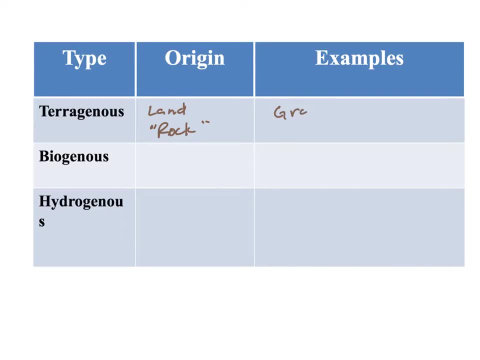 made up of rocks and minerals And that would be like a gravel or a mud sediment that you would find out there, And it's going to be made up of these minerals. The next is the biogenous. Remember, biogenous comes from life, And then this is going to be: